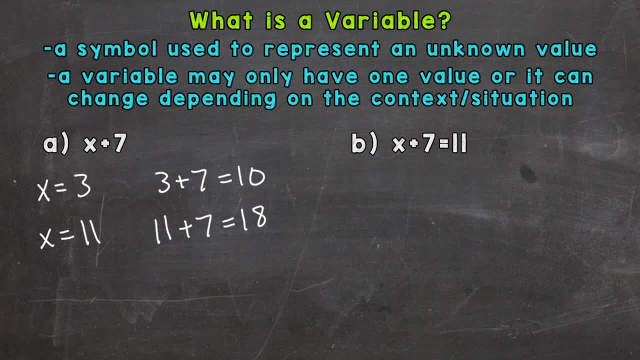 So again, in this situation the variable's value is not defined and a real world situation for that expression. we could say: we have someone that makes seven dollars an hour plus any tips they make. So do we know exactly how much they would make an hour? Not exactly, because we don't know. 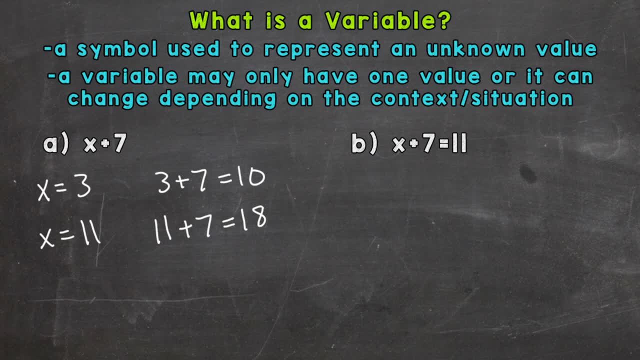 how much tips they'll make each hour, So that x will represent the unknown. Let's say they make three dollars in tips. Let's say they make three dollars in tips. Let's say they make three dollars in tips The first hour they work that day. Well, that three dollars plus the seven dollar hourly. 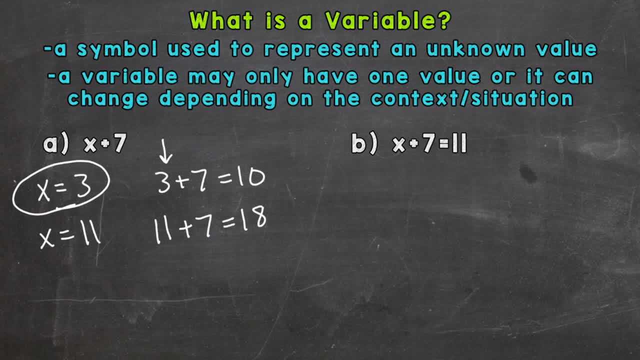 wage they would earn ten dollars that hour, Let's say the next hour. they earn eleven dollars in tips, right, So the variable's value is eleven. So we would have eleven dollars plus the hourly wage of seven dollars equals eighteen dollars for that hour. So again, a variable's value can change. 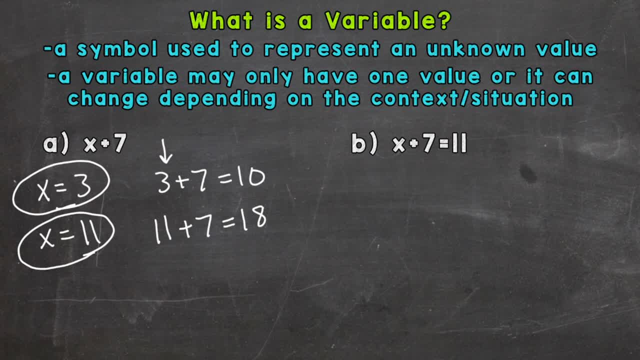 Now in situation b We have an equation there We have: x plus seven equals eleven. Now the value of x is defined. It has to equal one thing. So for example, here again x plus seven. We would solve this algebraic equation by getting the x by itself. So let's subtract seven from both sides. 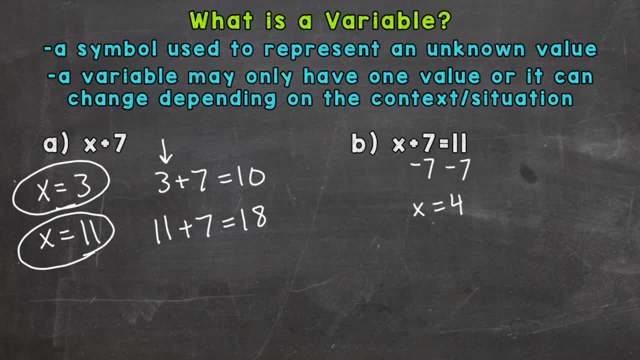 and we end up with x equals four. You can also figure that problem out using mental math. So x has to equal four. Four plus seven gives us that eleven. We can't say that x equals six here, Because if we plug in six we would get six plus seven equals eleven, which is not true. 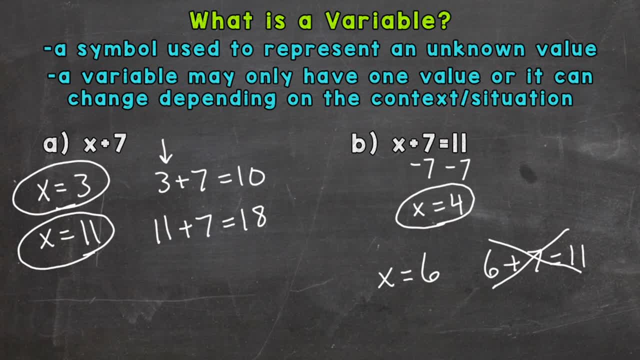 So in situation b we have an equation in which that variable has a defined value. It has to equal four there. So there are a few basics and kind of an introduction into variables. and remember, a variable is a symbol used to represent an unknown value and we went through one example where that value could change right. 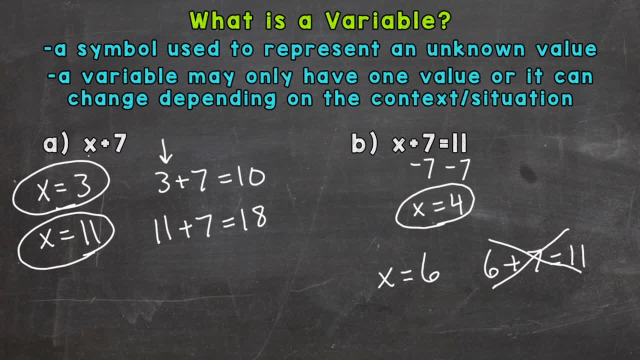 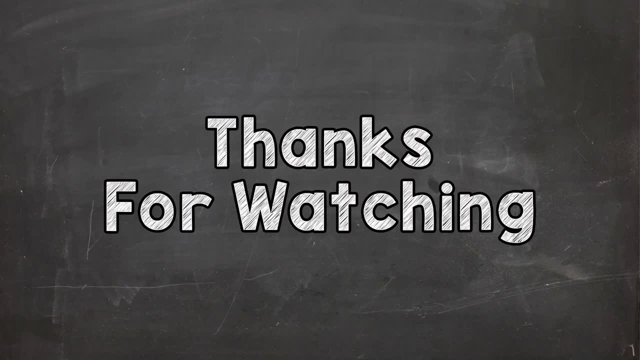 example a there and we went through one example- example b- where the variable had a defined or set value. so i hope that helped. thanks so much for watching until next time, peace you. 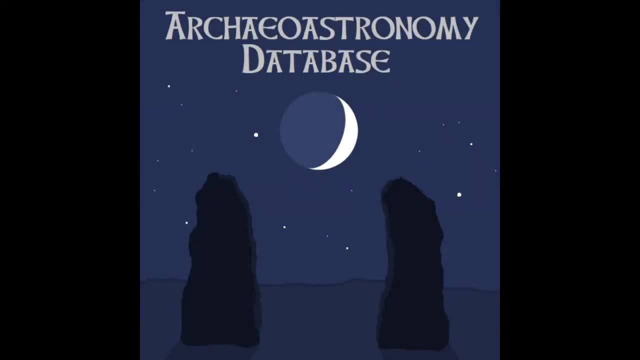 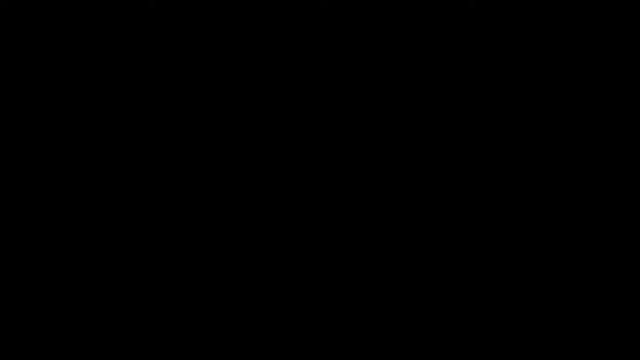 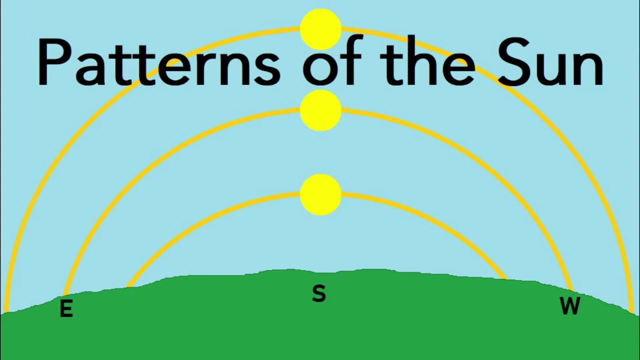 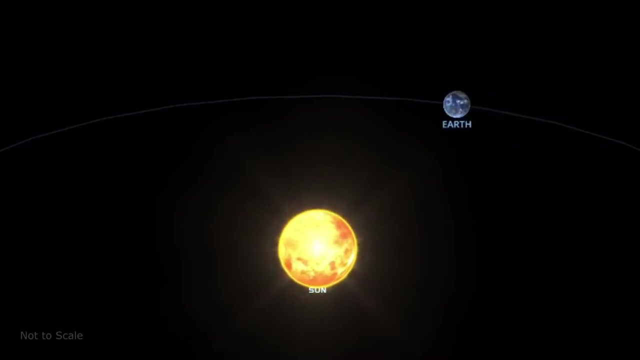 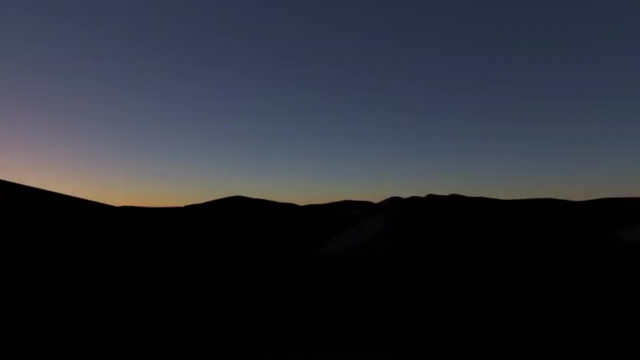 The Earth spins each day, as it orbits around the Sun once a year. However, from our point of view, on the surface of the Earth, it is the Sun that seems to move. Each day, it appears to rise, cross the sky from east to west and set below the horizon The place where 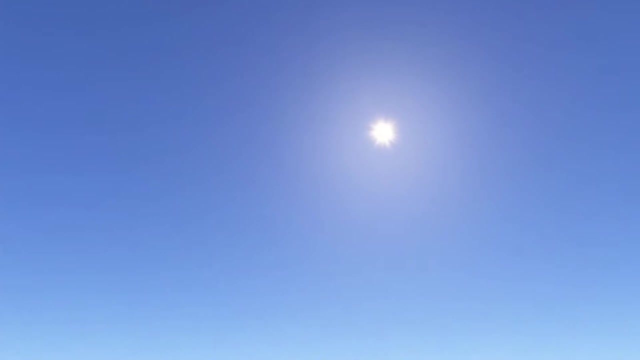 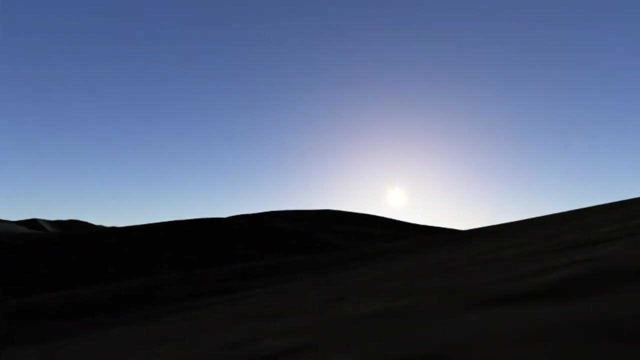 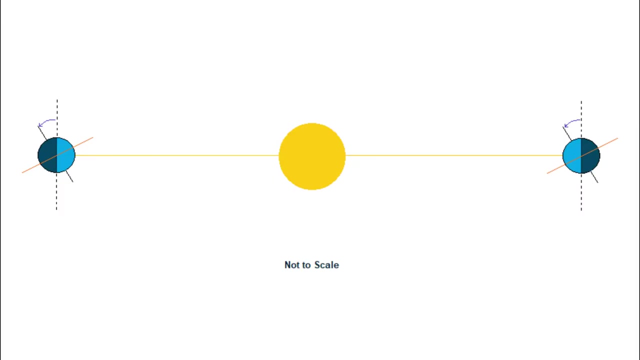 the Sun rises and sets the path it traces in the sky, and its position relative to the stars changes by a small amount each day, in a pattern that repeats over the course of a year. These changes happen because the Earth's axis is tilted relative to the plane in which it orbits the Sun. For half the year, the 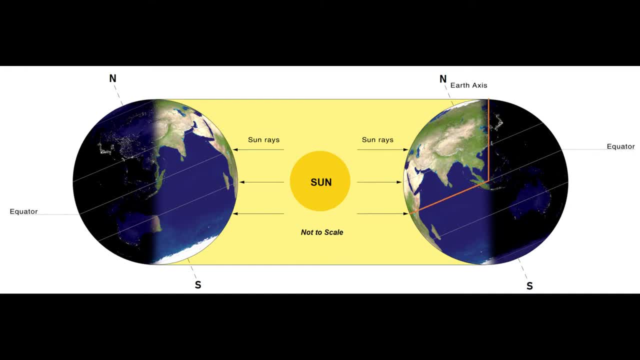 direction towards the Sun is centered more on the northern part of the Earth, and for the other half of the year it is the southern part that is oriented more directly towards the Sun. This also affects which parts of the Earth receive more or less direct sunlight. 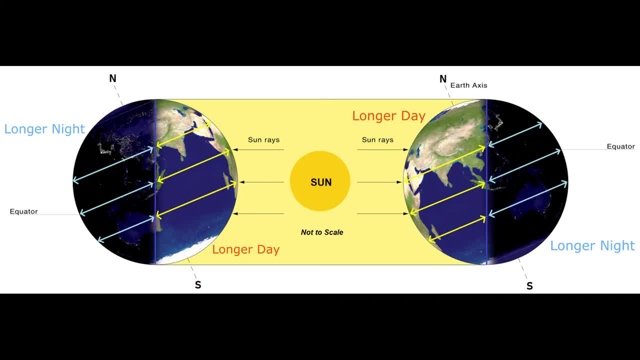 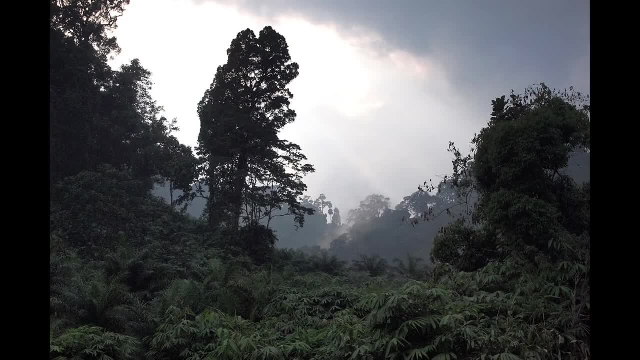 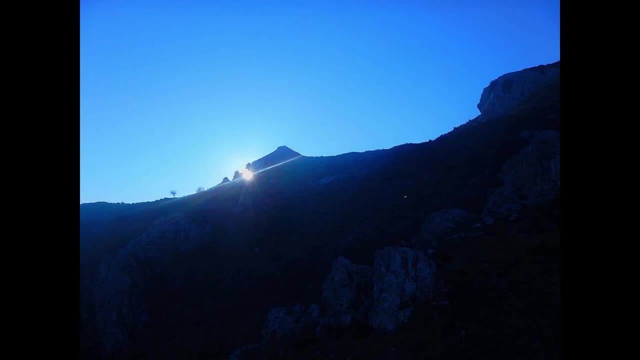 and greater or fewer hours of daylight. These variations produce seasonal changes in different parts of the Earth. The changes are less extreme towards the equator and more pronounced towards the northern or southern parts of the earth. The connection between these changes and the position of the sun in the sky.